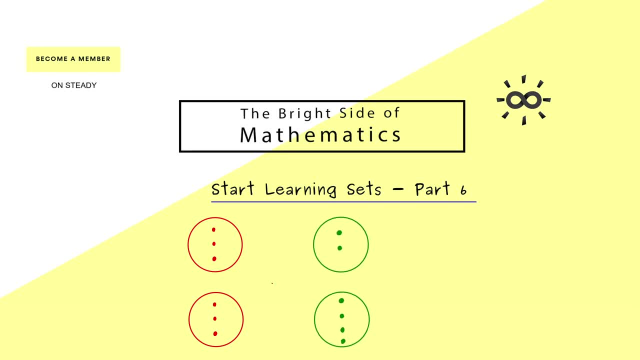 that you should really internalize them, And i think the best way to start with that is to look at these two examples here. So we have a set a on the left hand side and a set b on the right hand side. Now the map is given by these three errors, which means we send this element to this one. 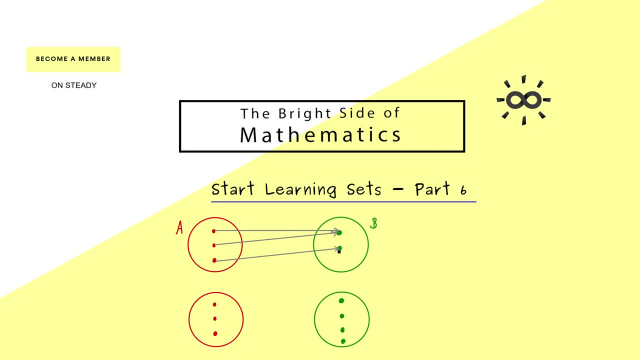 this one to the same and the last one to the last one in b. Well, since we hit the first element in b two times, we would say: this map is not injective. So you already see, the term injectivity should exclude something happening like this. Okay then let's look at the next example. 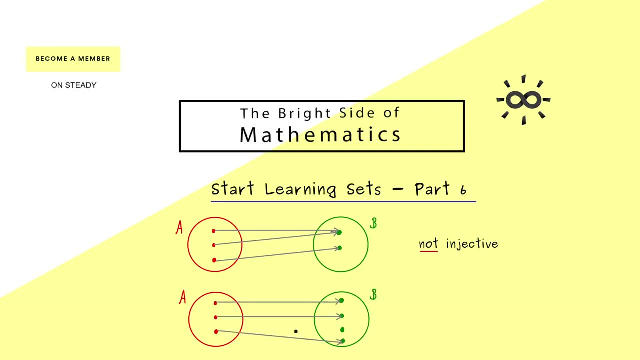 Where something different happens. As before, the map is just defined by the errors. and here we see: this element here is not hit at all. For this reason we call such a map not subjective. So you already see. subjectivity means that no element on the right hand side is left out. Okay, with these. 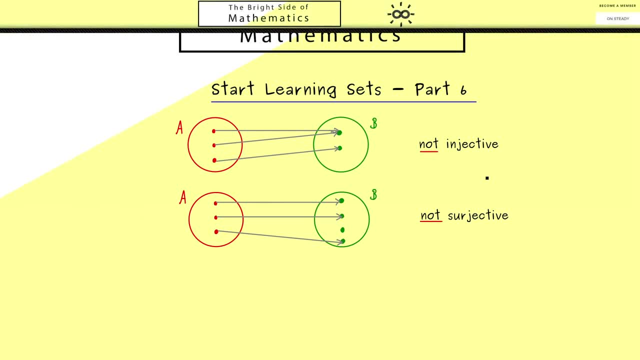 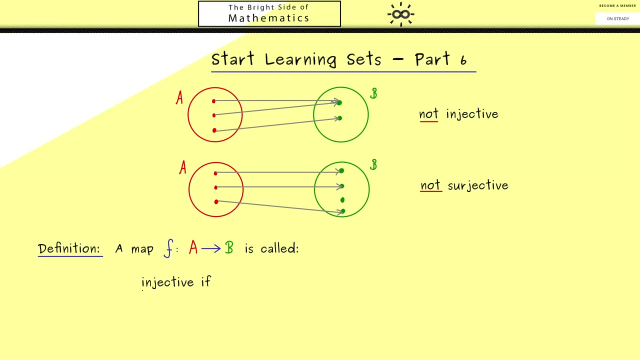 ideas in mind, we can go to the formal definition For this. let's fix a map f from a into a set b. Now the map is called injective. if for all x1, x2 in a, we have that if x1 and x2 are not equal. 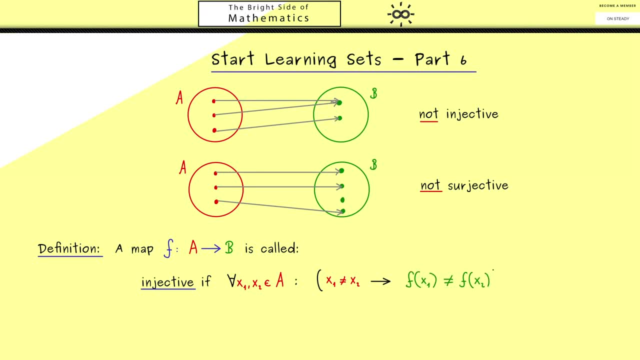 then this implies the two outcomes are also not equal. Looking back at the example from above, we see this: exactly forbids something like this. In a similar way we now can say: a map is called subjective if for all y in b there exists an x in a, such that f of x is equal to y. Also here we could look back at the example. 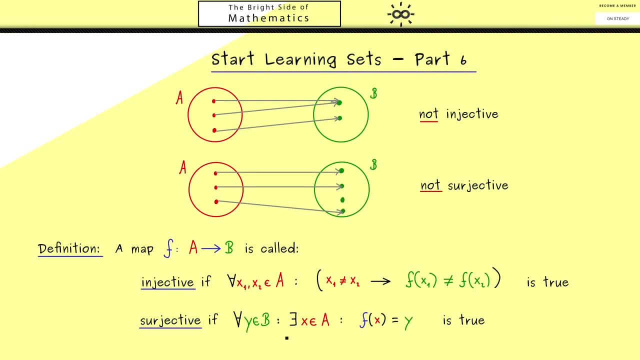 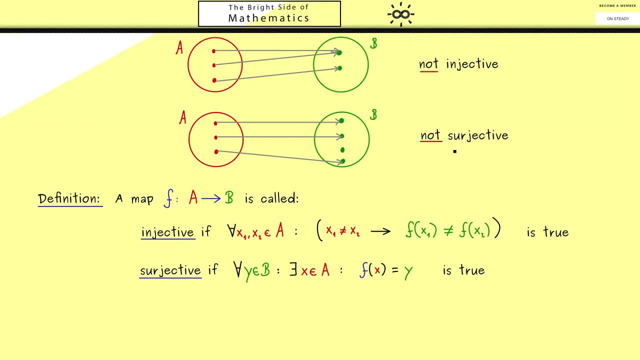 and see. something like this is not allowed. So for a subjective map, we can't omit any of the y's in b. Okay, so this is the definition of an injective or a subjective map. you really should know when you want to write down some proofs. However, to remember the terms, maybe the following is more helpful: 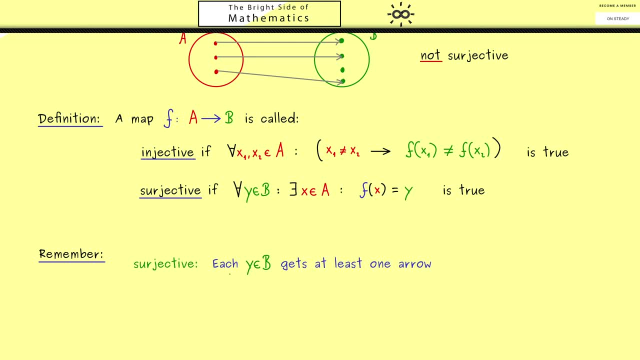 For the injectivity, please remember. it means that each y on the right hand side gets at least one arrow. So it's a target, it can't be omitted, but it could be hit multiple times. Therefore, at least one arrow reaches the y. Then for the injectivity, we know omitting is. 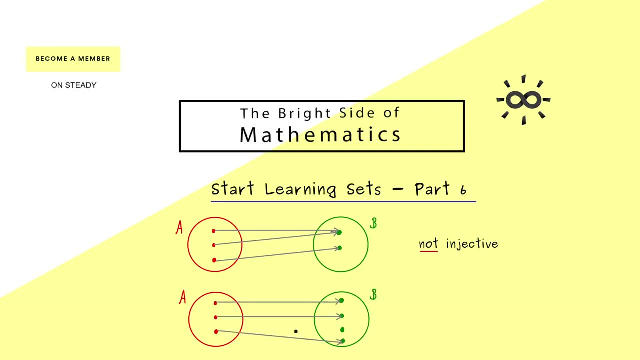 Where something different happens. As before, the map is just defined by the errors. and here we see: this element here is not hit at all. For this reason we call such a map not subjective. So you already see. subjectivity means that no element on the right hand side is left out. Okay, with these. 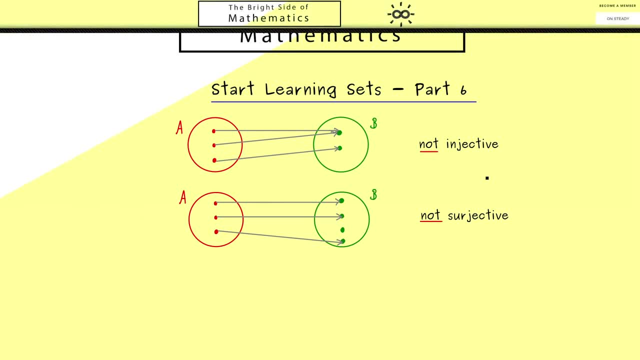 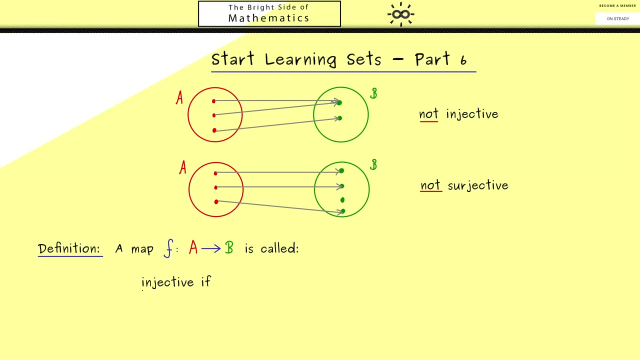 ideas in mind, we can go to the formal definition For this. let's fix a map f from a into a set b. Now the map is called injective. if for all x1, x2 in a, we have that if x1 and x2 are not equal. 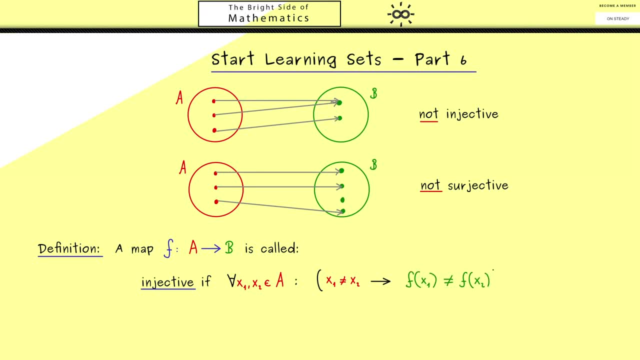 then this implies the two outcomes are also not equal. Looking back at the example from above, we see this: exactly forbids something like this. In a similar way we now can say: a map is called subjective if for all y in b there exists an x in a, such that f of x is equal to y. Also here we could look back at the example. 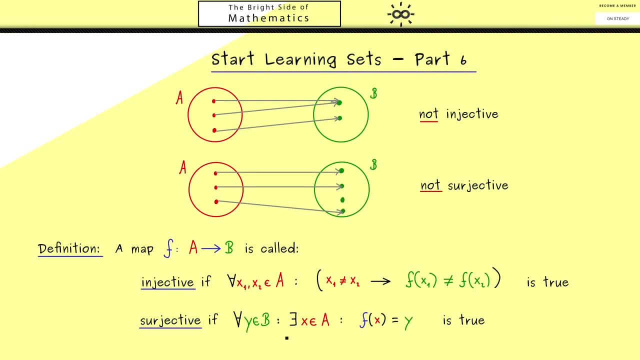 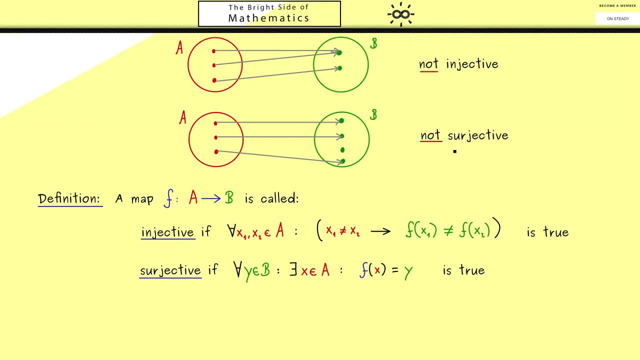 and see. something like this is not allowed. So for a subjective map, we can't omit any of the y's in b. Okay, so this is the definition of an injective or a subjective map. you really should know when you want to write down some proofs. However, to remember the terms, maybe the following is more helpful: 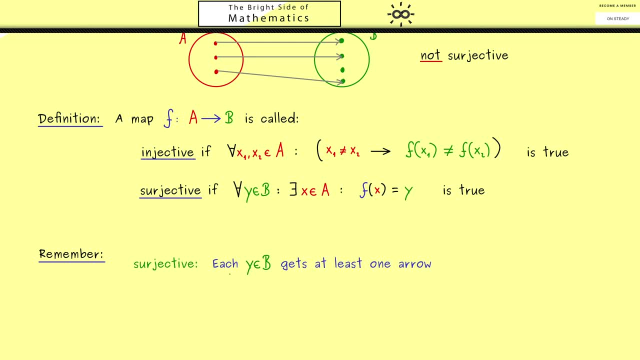 For the injectivity, please remember. it means that each y on the right hand side gets at least one arrow. So it's a target, it can't be omitted, but it could be hit multiple times. Therefore, at least one arrow reaches the y. Then for the injectivity, we know omitting is. 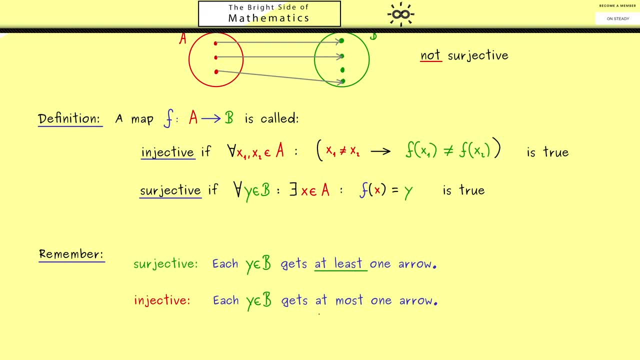 not a problem, but hitting multiple times is a problem. So here we know, each y gets at most one arrow. Therefore, now you see, both things together is a very nice property. These two concepts are Binary Placement Mechanisms, and there are actually words that would be quite. 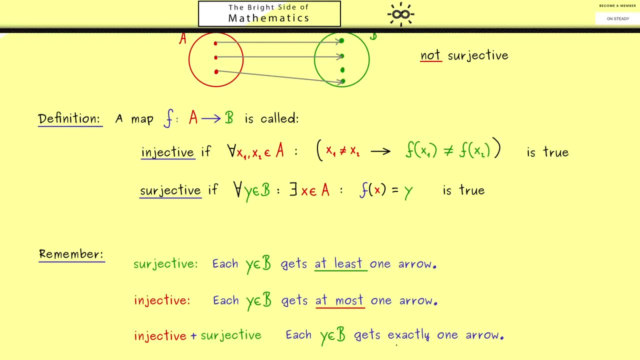 useful in the future. To make this simplest way to write sheets of people on a 1up or 1d of sides, you go over to the left hand side of a part of our surface For this section. you can skip to 4.. 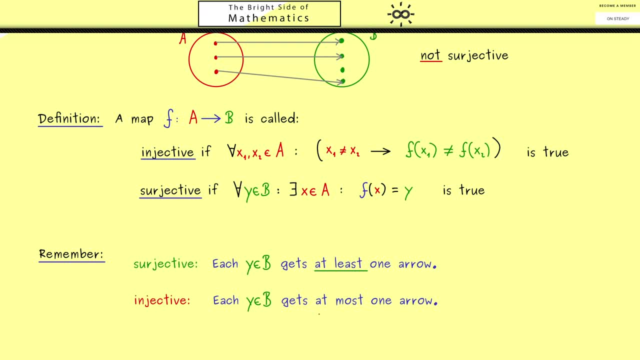 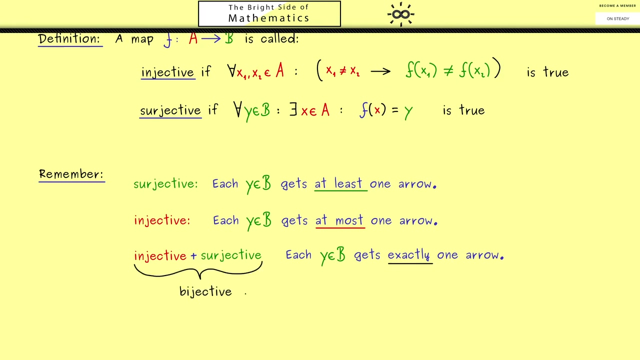 not a problem, but hitting multiple times is a problem. So here we know, each y gets at most one arrow. Therefore, now you see, both things together is a very nice property. Becuase, the insertion is very good because both elements have the same scale And we have a new name for this property. 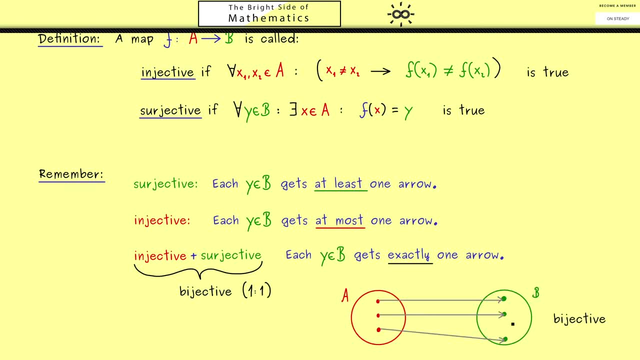 We call it a bijective map. Now, such a bijective map gives us truly a one-to-one correspondence between the two sets. So if we take an element, no matter from which side, Then there is exactly one connection to another element on the other side. Therefore, a bijective map can also be read from the right-hand side to the left-hand side: movie CL personaje and all ejec黄 cross Entoncesよね. 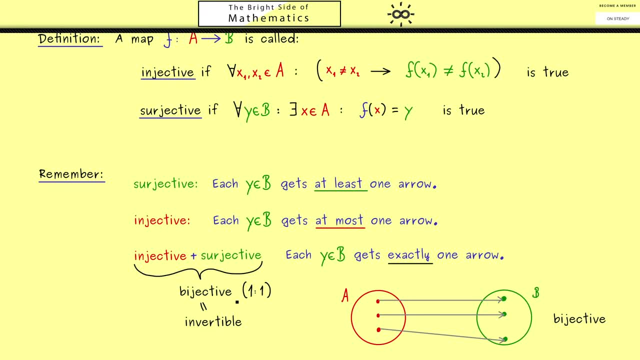 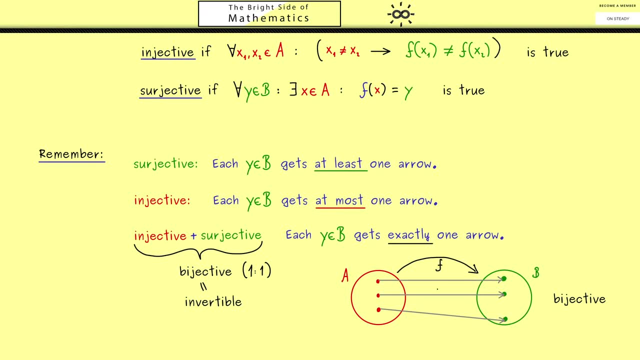 inside Hence for maps. one can also say bijective just means invertible In the picture. you can visualize that as the map f, that goes from a to b, and then the inverse map we read from right to left. so it's a map from b into a and it's 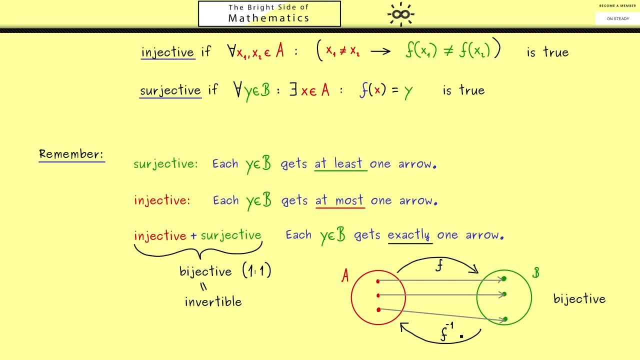 denoted by f to the power minus 1.. It's the same notation we use for the pre-image, but don't get confused here. in fact it denotes a new map. In both cases the notation makes sense and it fits together in the end, as we will see. but 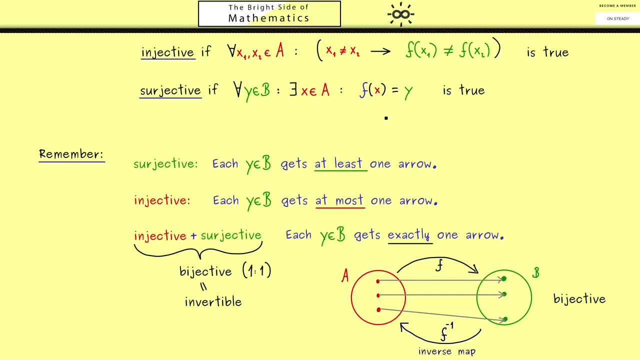 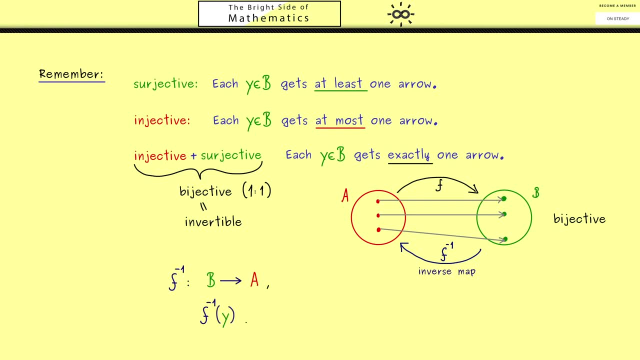 please remember they denote two different things. Okay, here we call f to the power minus 1 the inverse map, and soon I will tell you why the name makes sense. Okay, for the sake of completeness, let's write down the definition of this inverse map. so it's a map from b into a, and f to the power minus 1 of y is 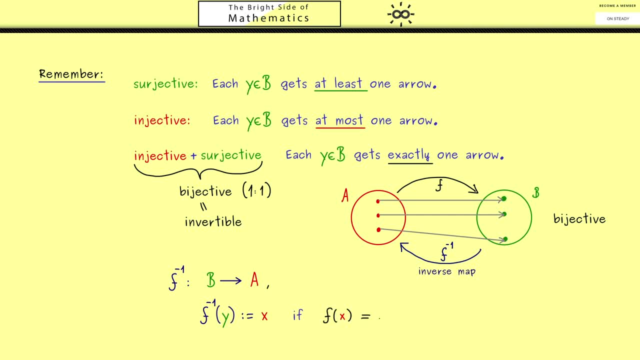 defined as x if f of x is equal to y. So you see that the inverse map is a map from b to a and f to the power minus 1 of y is defined as x if f of x is equal to y. So you see that the inverse map is a map from. 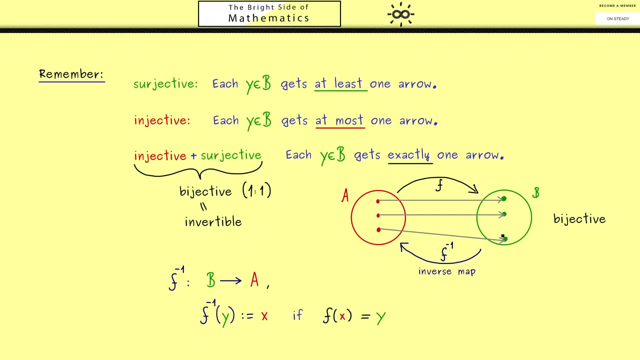 b to a and f to the power minus 1 of y is defined as x if f of x is equal to y. So this is exactly what we mean when we say we read the map from right to left. However, I think it's better to understand when we look at an example. So 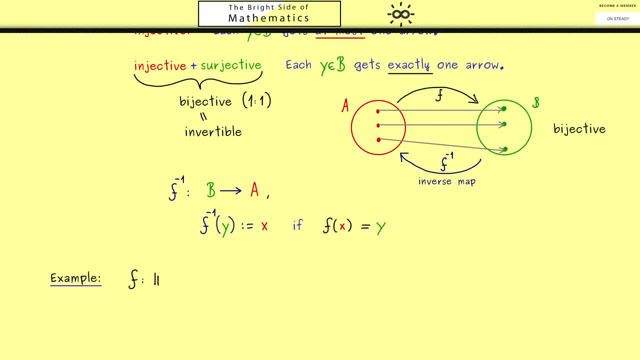 let's take the function f to be a map from the natural numbers into the square numbers, and now we simply map x to x squared And now you should see, the map is in fact injective and we also hit all the elements on the right hand side. 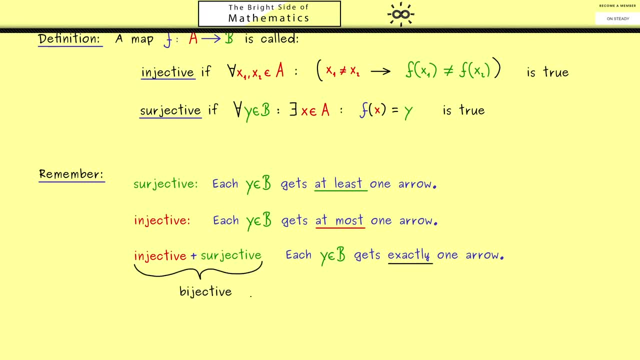 This is same as being responsible for the two points which are stomach a. just read thecht unn. Now we suddenly know that such a bjective map can also call exactly one Alabama還有 left hand side. Hence for maps one can also say: bijective just means invertible. 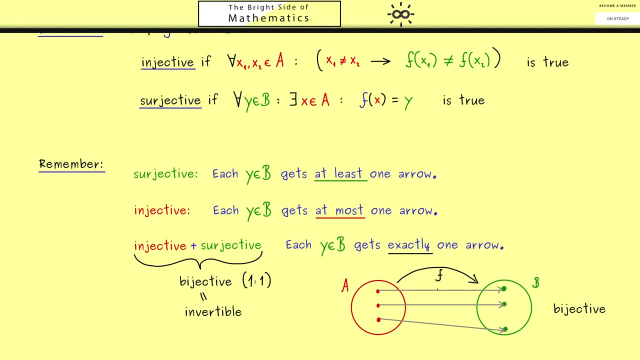 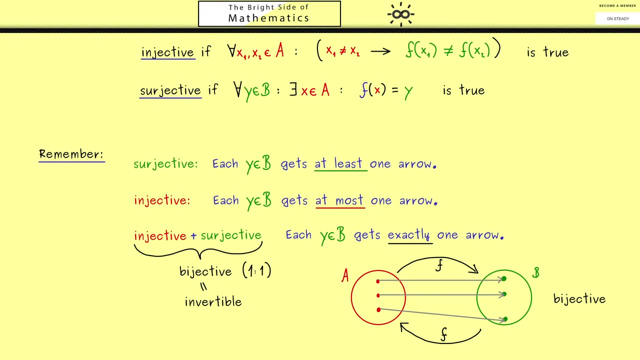 In the picture. you can visualize that as the map f, that goes from a to b, And then the inverse map we read from right to left. So it's a map from b into a and it's denoted by f to the power minus one. 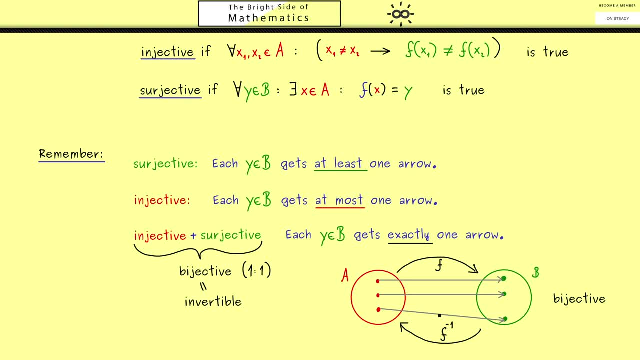 It's the same notation we used for the pre-image, but don't get confused Here. in fact it denotes a new map. In both cases the notation makes sense and it fits together in the end, as we will see, but please remember they denote two different things. 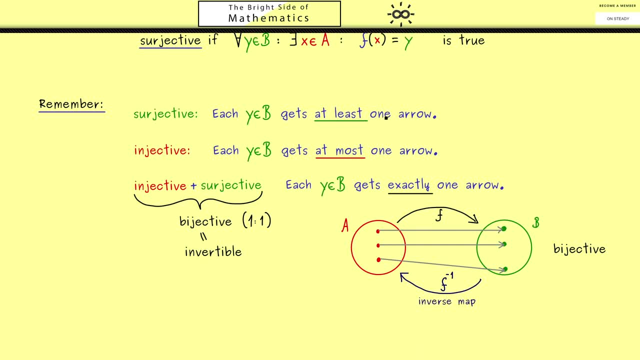 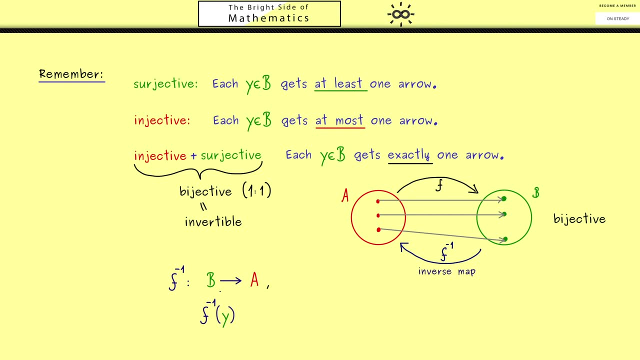 Ok, here we call f to the power minus one the inverse map, and soon i will tell you why the name makes sense. Ok, for the sake of completeness, lets write down the definition of this inverse map. So it's a map from b into a, and f to the power minus one of y is defined as x if f of x is. 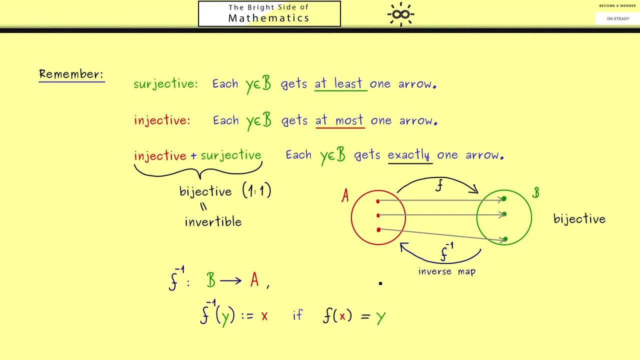 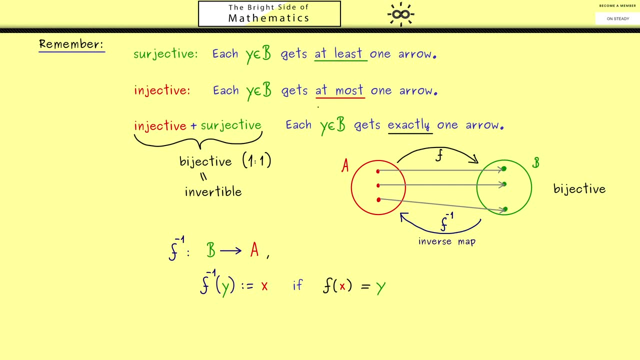 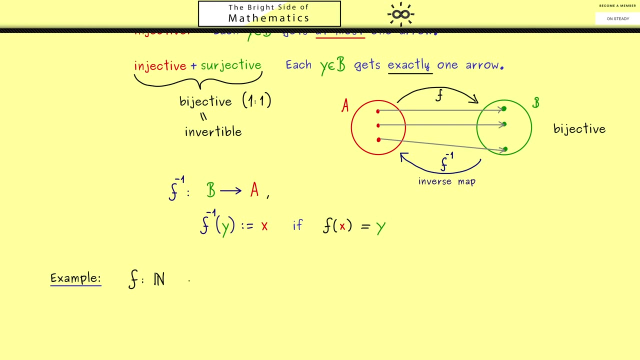 equal to y. So you see, this is exactly what we mean when we say we read the map from right to left. However, i think it's better to understand when we look at an example. So lets take the function f to be a map from the natural numbers into the square numbers. 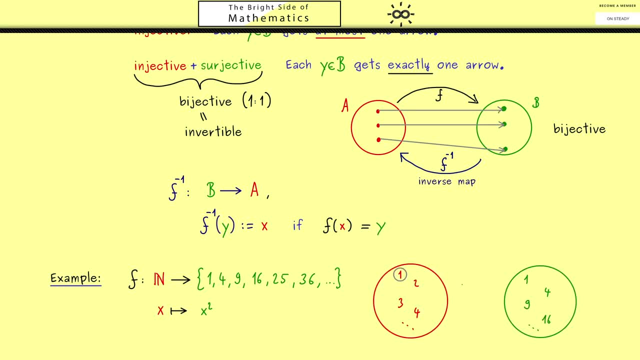 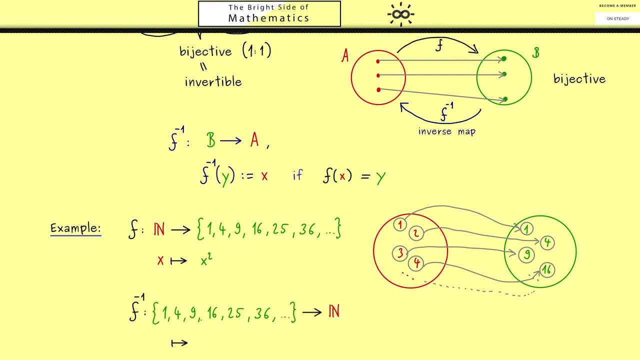 And now we simply map x to x squared, And now you should see, the map is in fact injective and we also hit all the elements on the right hand side. So the map is also subjective. Ok, But we have a bijective map such that we can write down the inverse map. 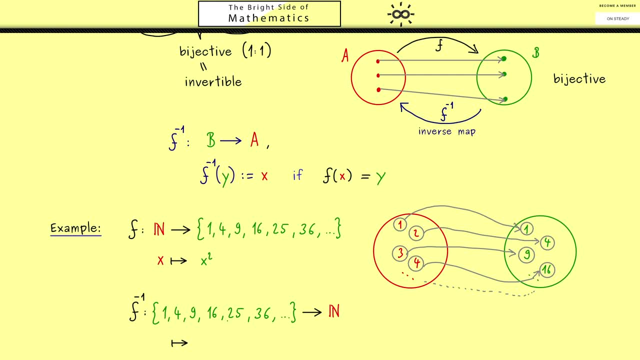 For it, the roles of the domain and codomain are exchanged, And now we look at an element in the green set, So lets call it y, And in order to get to the correct element in the red set, we have to take the square root. 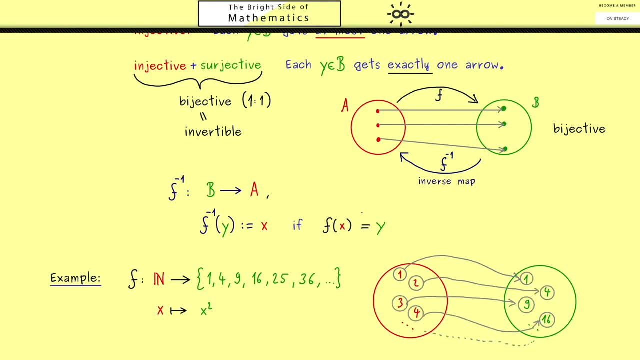 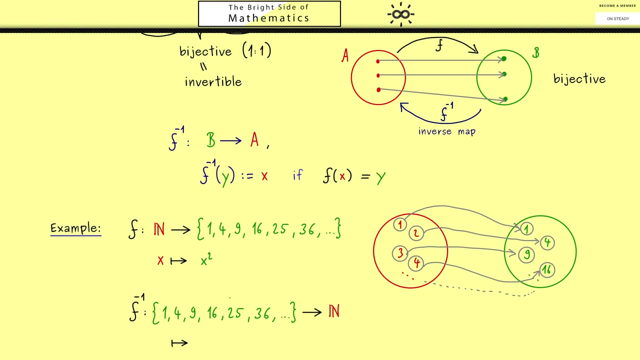 so the map is also subjective. In other words, we have a bijective map such that we can write down the inverse map For it. the roles of the domain and codomain are exchanged, and now we look at an element in the green set, So let's call it y, and in order to get to the correct element in the red, 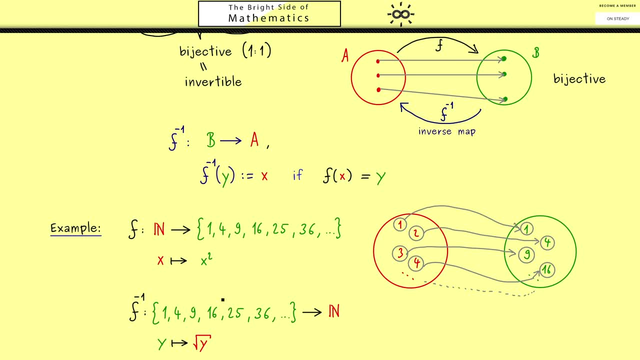 set. we have to take the square root. Okay, maybe that does not surprise you so much, but here you see the idea how we define new symbols and new operations in mathematics. Therefore, the terms injectivity, subjectivity and bijectivity comes in a lot in mathematics. With this, we will use the next video to talk a. 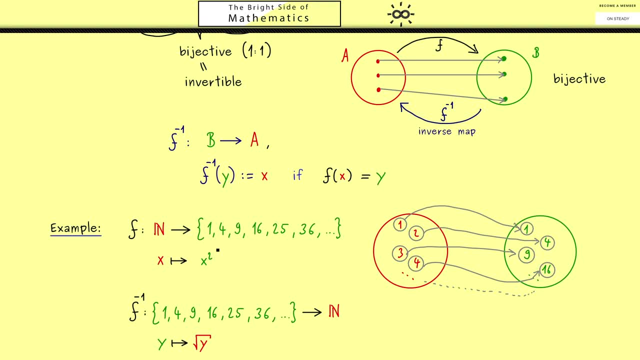 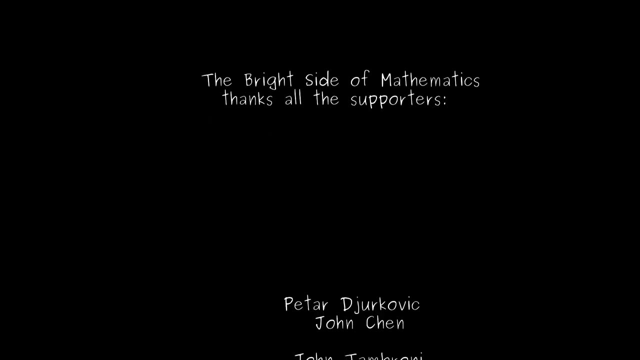 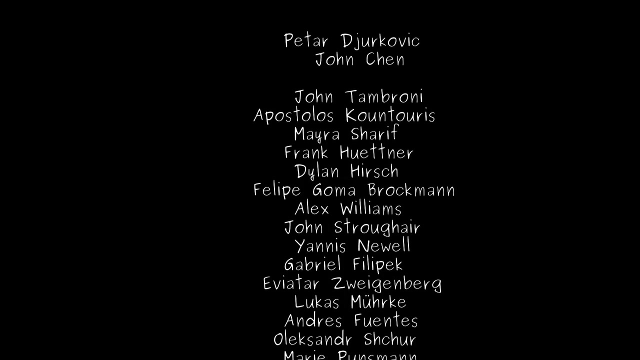 little bit more about maps, but after that we will finally start defining the numbers, So I hope I see you there and have a nice day. Bye. Subtitles by the Amaraorg community. 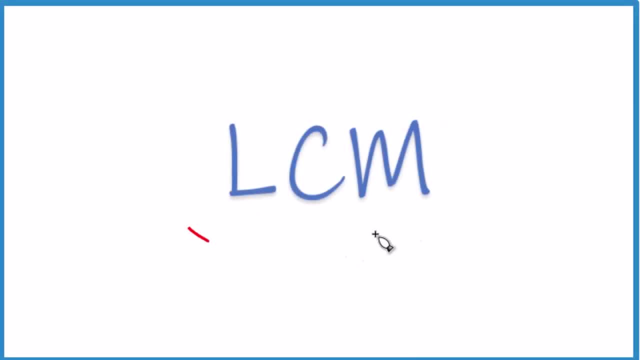 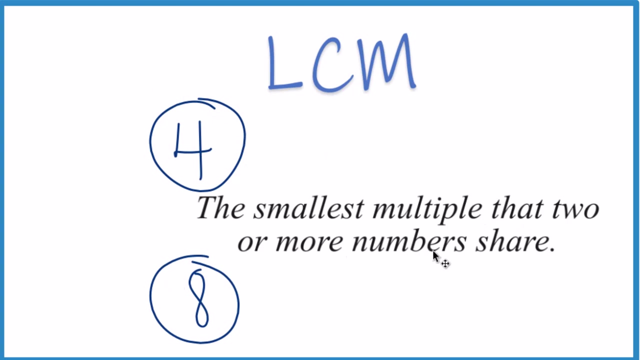 Okay, let's find the least common multiple, the LCM for 4 and 8.. So how do we do that? I like to think of the least common multiple as the smallest number, the smallest multiple that these two numbers- 4 and 8, share. So they both go into it evenly and it's the 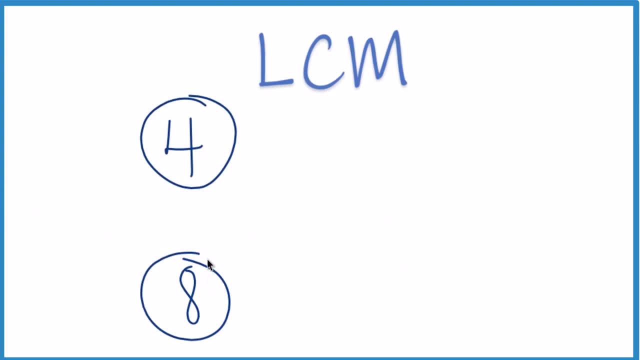 smallest one. So what we do, we'll find the multiples of 4 and of 8, look at the common multiples and choose whichever one is least. I like to start with the bigger number. That usually makes it a little bit easier. So we could say 8,, 16,, 24, but I can already see. 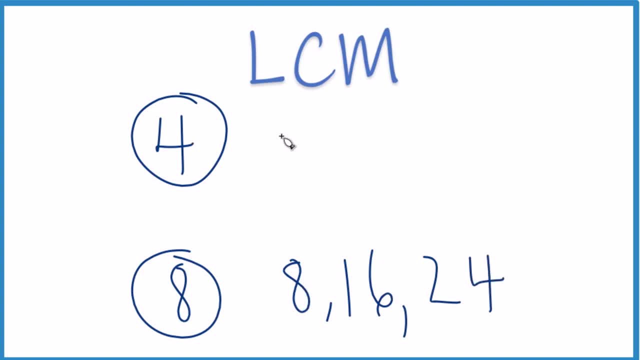 that 8, 4 goes into 8 evenly. So if we write the factors for 4,, 4,, 4 plus 4 is 8, and there it is. That is our common factor. It's the first one, so it's the smallest one, and that's. 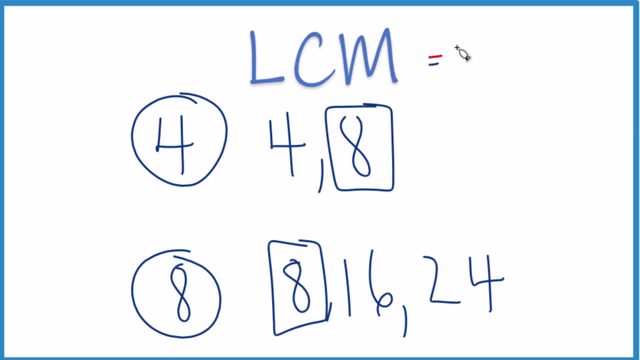 our common factor between 4 and 8.. That's the LCM. You could find the factors by saying: 1 times 4 is 4,, 2 times 4 is 8,, 3 times 4 is 12, and.